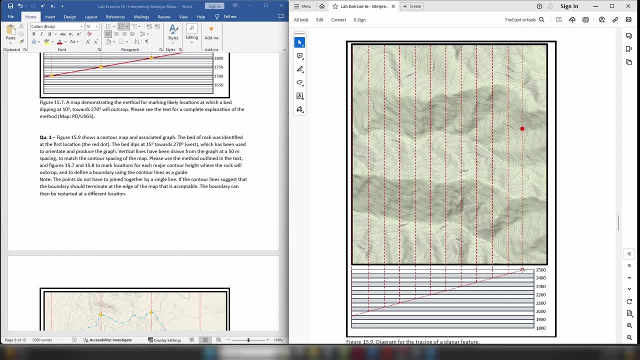 So okay. so on our graph we've drawn our starting point at 2500 meters above sea level, which matches the elevation. So this is the elevation of our known location. We know our layer of rock has a dip of 15 degrees and we know it is dipping to the west. So we know our layer of rock is dipping 15 degrees. 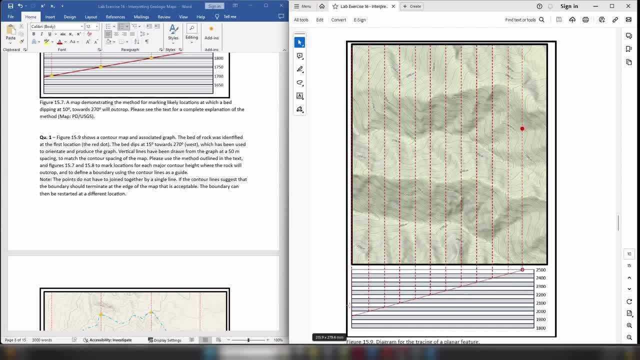 towards the left hand or western side of our graph and map. So you can see that I have drawn vertical lines coming off this diagonal line here representing our layer of rock, and I have done that at 50 meter increments. So, just like in the worked example, what you're going to do is you are going to mark every location. 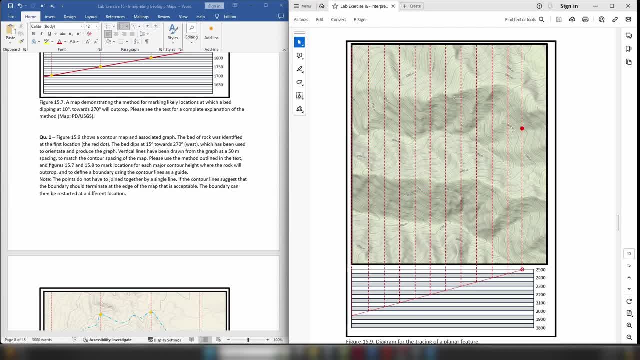 where the vertical line here crosses a contour line of the same height. So in the case of this 2500 meter line, you can see it's coming up like so and we know that this contour line here is the 2500 meter contour line. So we know that this contour line here is the 2500 meter contour line. 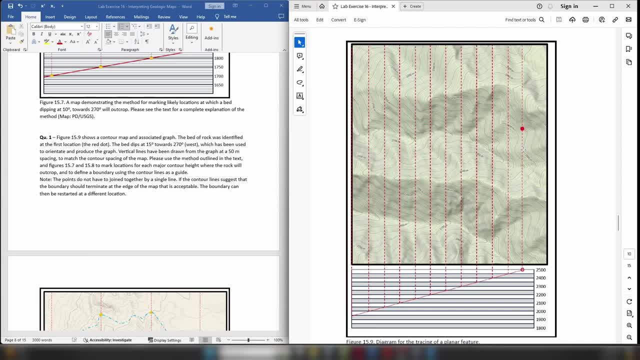 So if we follow it around, it comes around, it comes really close right there, then it comes around here and then eventually it crosses the 2500 meter line right here. So we're going to have to draw another point right there. We're then going to continue tracing the 2500 meter line. We're 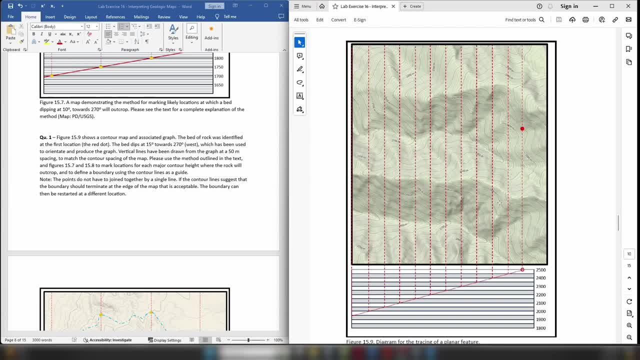 going to come around here, then we're going to come back, we're going to keep going and then we are crossing the line There as well. So we have another point where our 2500 meter contour is crossing this vertical line, So we're going to make another point there. So, remember, you have to make a mark every time your 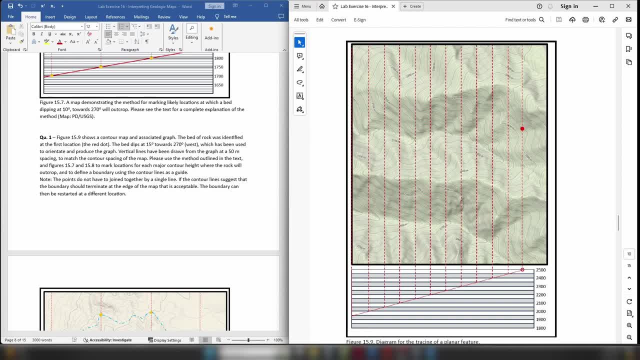 contour line of the same height crosses the matching vertical line, And of course these are in 50 meter increments. So this one's going to be the 2450.. This one's going to be the 2500 meter, and this one's going to be the 2400, etc. And so you are going to have a lot of points on this map. 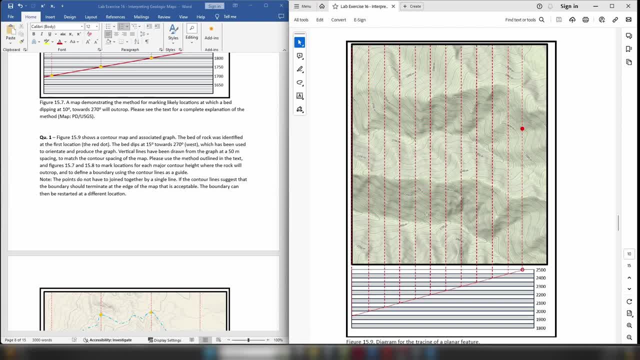 because this is quite a complicated topographic map. Now you will notice it's quite obvious that they've actually helped you a little bit because they've shaded this map. You clearly have a valley running through here. You have another valley running through here, Then you have a ridge of. 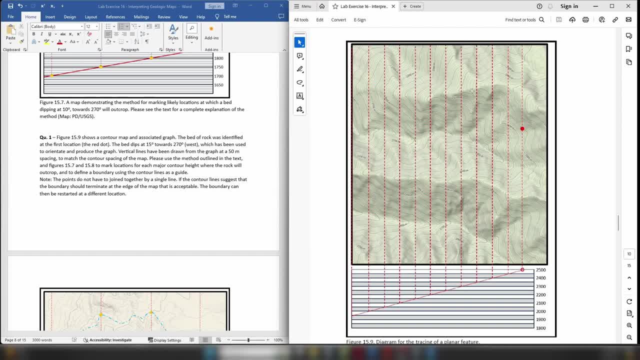 high ground running up here, Another ridge of high ground running up here, And then you have several smaller valleys running up here, And then you have a ridge of high ground running up here, Valleys there and there located on the north side of this ridge, And then you have some smaller. 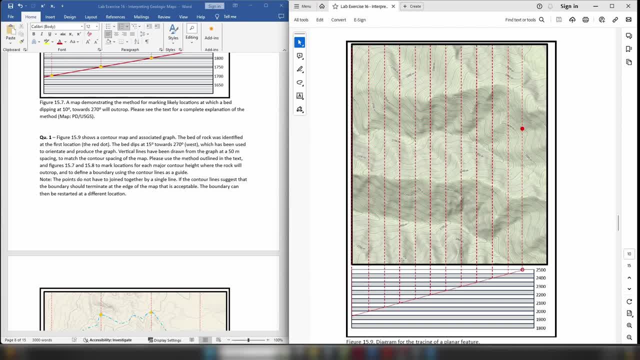 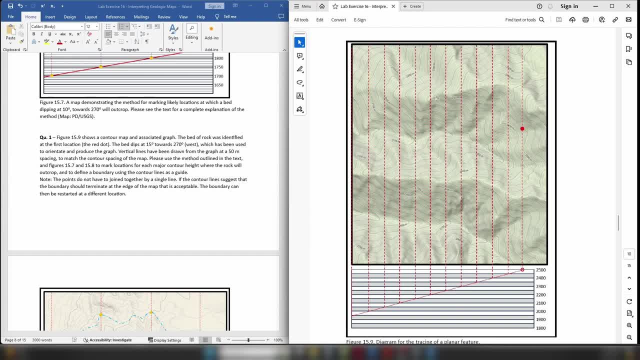 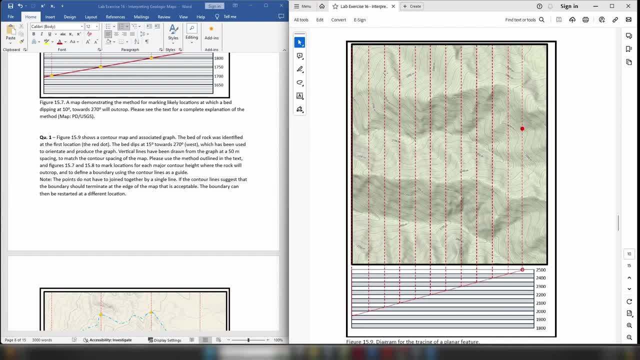 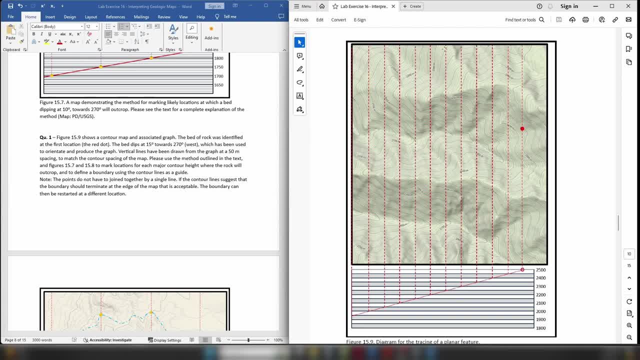 come to this point, you start turning around. this is your final point over here, and then you have to draw a line straight over to the next point over here. don't do that. follow the topography. so in this case your line would come round and then it's going to follow the topography to the north. 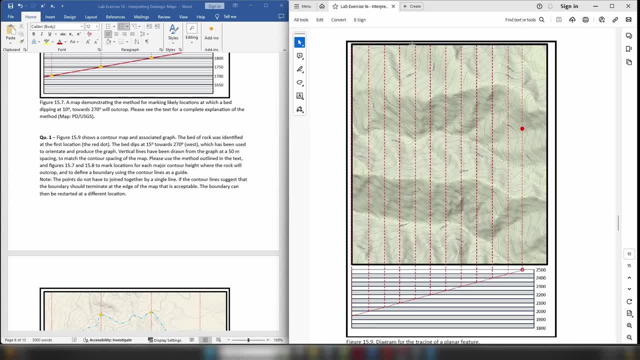 and then your line is going to restart at another point along the edge of the map, and then it's going to start following the topography over in that area as well, and so once you've done that, you are going to have marked out the probable locations where this layer of rock could outcrop. 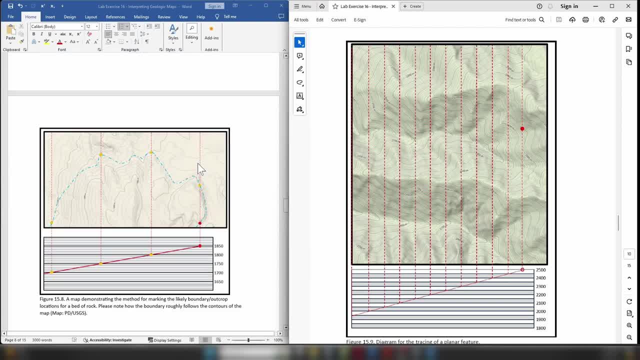 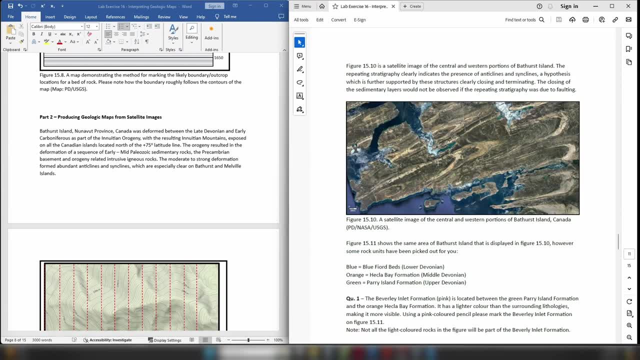 and that will be the end for part one. question one: okay, so for part two we are going to be looking at satellite imagery. so bathurst island is the area which is shown in the satellite image and this is in nunavut province in canada. so this is one of these islands to the north of mainland. 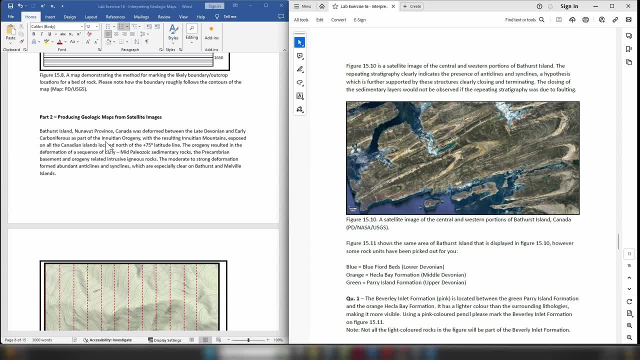 canada. so it's one of these areas that is obviously very, very cold and quite difficult to get to, so this is an area where satellite analysis is extremely helpful for geologists. so this particular area was deformed during the inuitian orogeny and this produced the inuitian 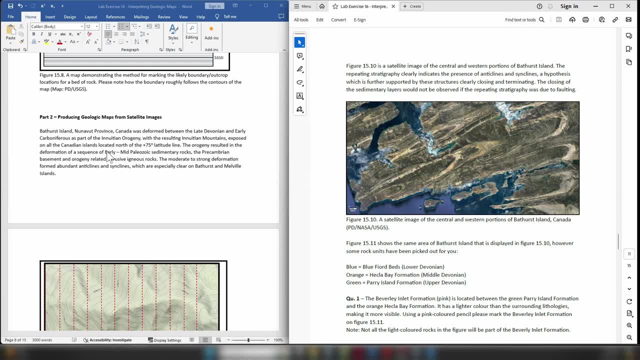 map. the defamation produced as part of that mountain building event is observed in rocks on these islands above 75 degrees latitude. so once you're above that latitude line, you're going to see the rocks on those islands showing signs of defamation related to the inuitian orogeny. now, the orogeny itself occurred between the late devonian and early carboniferous and in the inuitian orogeny itself occurred between the late devonian and early. it led to the deformation of a sequence of rocks that date from the early to mid paleozoic, so the defamation affected a package of rocks that contained rocks dating from the cambrian. the ordovician, the silurian and the majority of the devonian as well. so both early, middle and late devonian rocks which were laid down before defamation began were affected by the inuit fan orogeny. now, if i just zoom in over here on the right, you can see the inuitian orogeny. 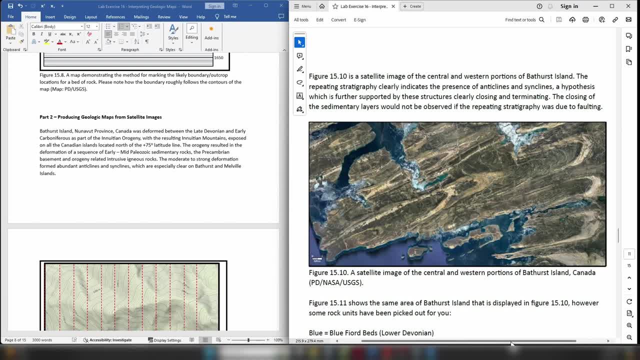 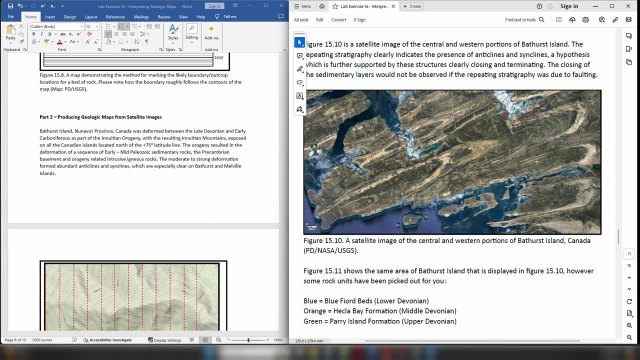 into the division between the second and fourth generation been stretched into a flourishing right, you can see that the rocks exposed do have a rather distinctive pattern to them. In fact, if you look over here, on the right especially, you can see you have a bit of a sawtooth or zigzag. 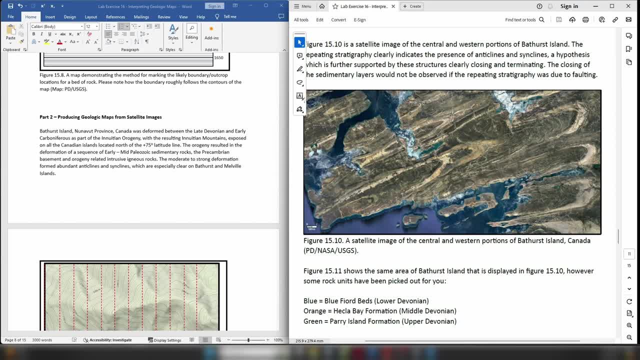 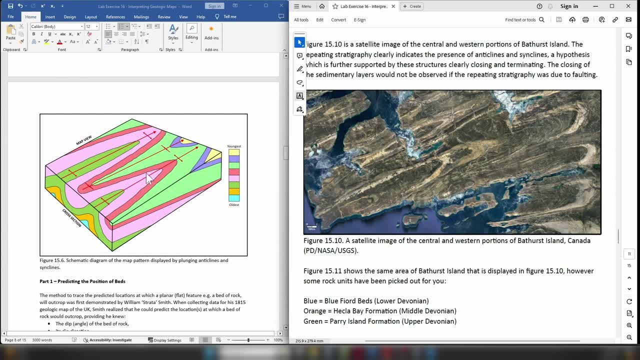 pattern which is highly reminiscent of one of the block diagrams that we saw earlier. So if I just come up here, it looks a lot like this. There's that sawtooth pattern on the diagram and you can see the same sawtooth pattern here as well, So straight away we can see that the rocks have been. 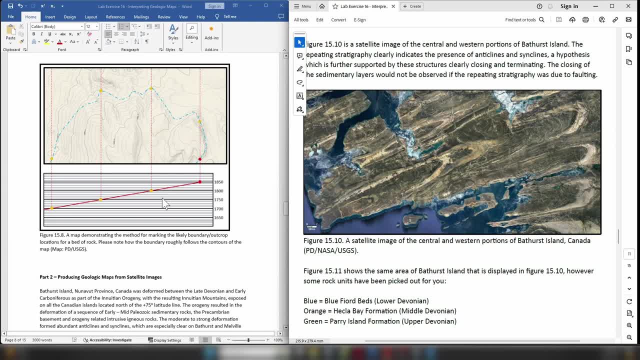 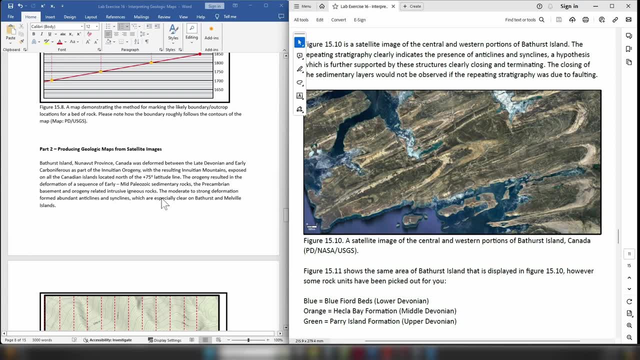 deformed, because we can obviously pick out geologic structures which are related to deformation in our satellite photograph and we can also begin to already make an assumption that these structures that we're seeing are quite likely to be anticlines and synclines. The reason that I say 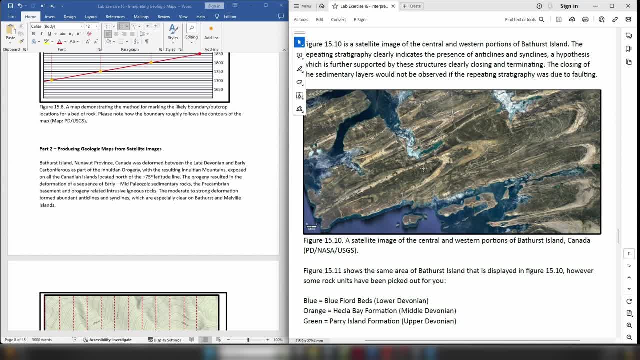 this is because I'm not sure if you can see it. but I'm not sure if you can see it, but I'm not sure, because if this repeating of the same layers of rock was the result of faulting, we wouldn't be getting this zigzag sawtooth pattern. So this is a strong indicator that what we're looking at are. 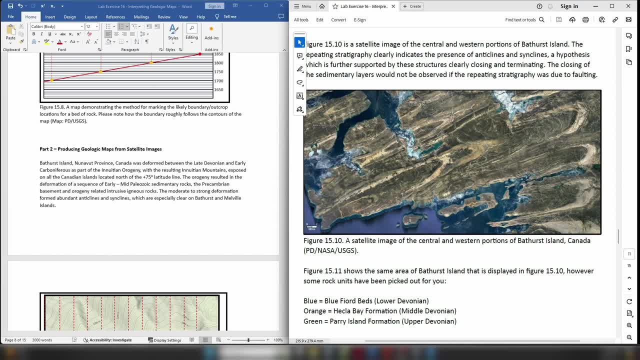 anticlines and synclines, So the deformation that we see in the satellite image isn't just limited to Bathurst Island. There are also very good examples of these anticlines and synclines on the nearby Melville Islands, But there are also several other islands located in the area which show similar anticlines and 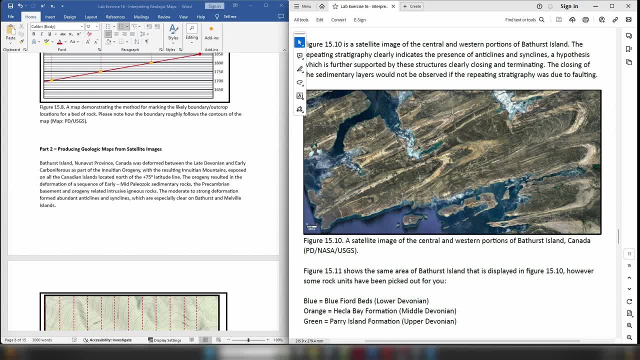 synclines. Now, when they are outcropping on these islands, these anticlines and synclines all show the same approximate orientation, which is a strong indicator. they were all formed by the same event, and the fact they are spread out over such a large area, so between several islands, suggests that 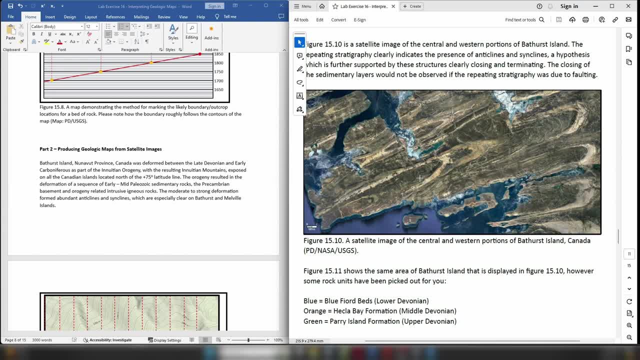 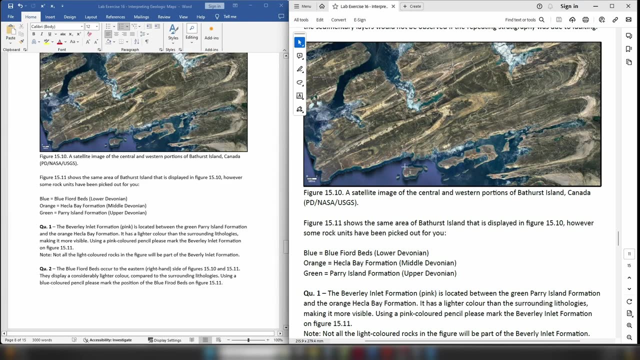 whatever this event was, would have been quite large. So it's very likely that the deformation of the satellite image is related to a relatively major orogenic event. So when we look at our satellite image we can quite clearly see that there are some layers of rock that 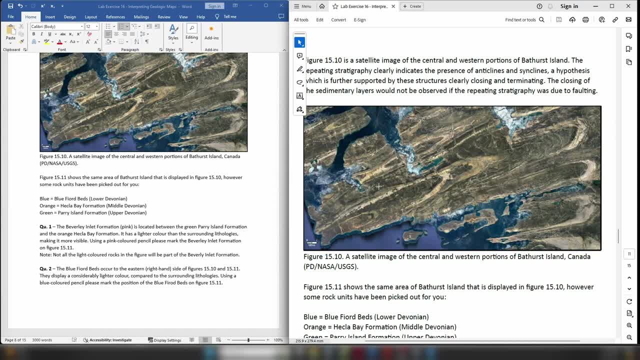 have a very distinct colour to them, so they stand out when compared to the surroundings, and some of these rocks are also obviously forming topographic highs, which would suggest they are harder than some of the other layers of rock which are exposed. So, for instance, we can quite clearly see that we have this line of lighter coloured rock coming around here, and so that's quite easy to pick out based on the colour. 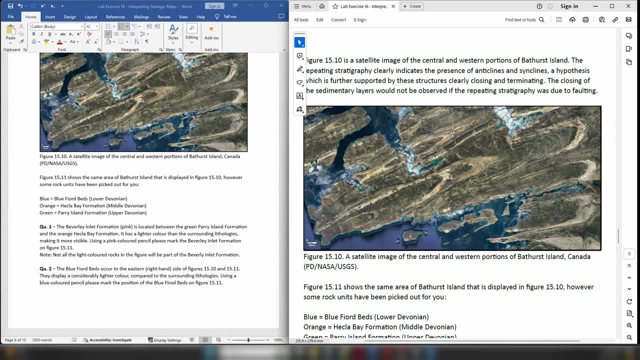 But you can also see that it does appear to be forming quite an obvious topographic high, which would suggest it's more resistant to erosion when compared to this layer of rock here. You can also see we have another layer of rock here and this one has a slightly different colour. it's kind of more of an orange, brown kind of. 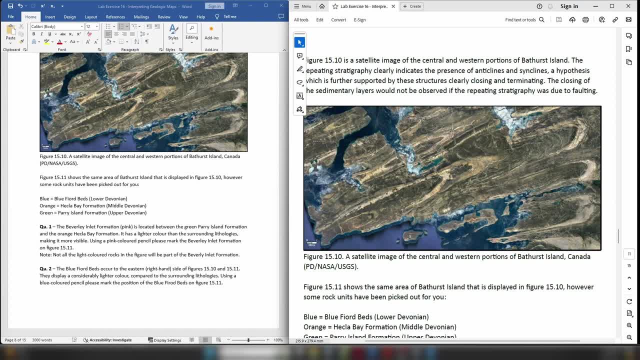 colour right here, and this too is forming topographic highs, so it's obviously slightly more resistant to erosion than these rocks here. Now, the rocks that are in these areas here, we can't really identify them, we can't really classify them, because they are covered by vegetation. 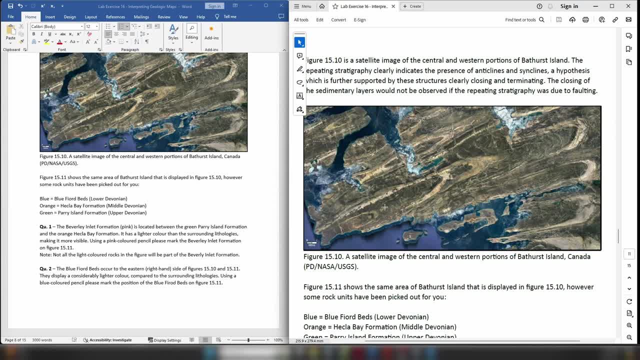 and this vegetation just gives them a kind of green-brown appearance. so, even though the rock here and the rock here are probably different layers of rock, We can't get a solid雞屑 床 andêm be certain, because we can't see them, and so the only way to be certain would be to send a geologist. 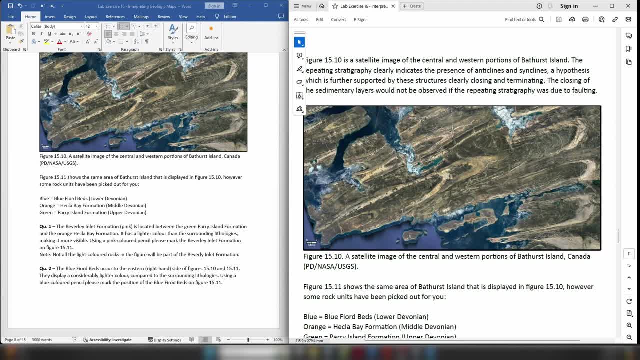 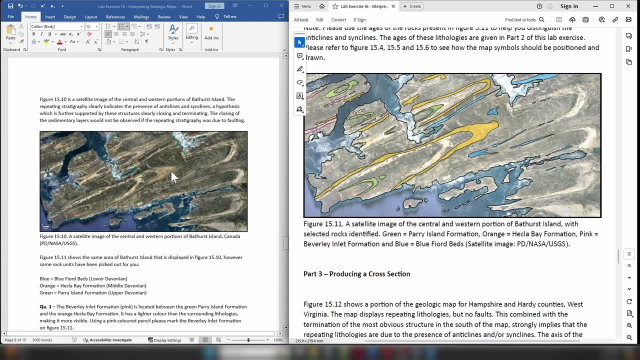 to the area to collect samples. So I'm just going to come down to the next figure, and in this figure you are going to see the satellite image that we were looking at a moment ago. but you will see that I have begun to pick out some of these layers of rock based on the colors that can be seen in the 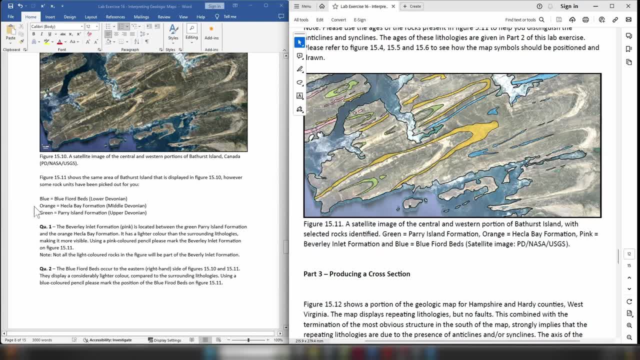 satellite image. So if we look over here on the left, you will see that there are three layers of rock which I've picked out. So in blue, so these layers- here we have the blue fjord beds and these are lower Devonian in age. And in orange, so this color, here we have the Hekla Bay formation. 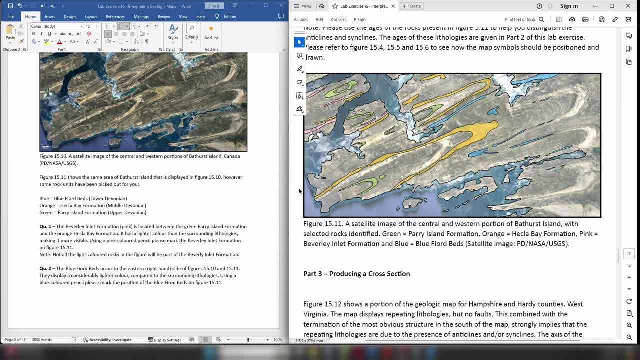 and this is middle Devonian. and then in green, here here, here and over there, We have the Parry Island formation and this is upper Devonian. So the blue rocks, the rocks I've picked out in blue, should I say, are going to be the oldest and the green rocks are going to be 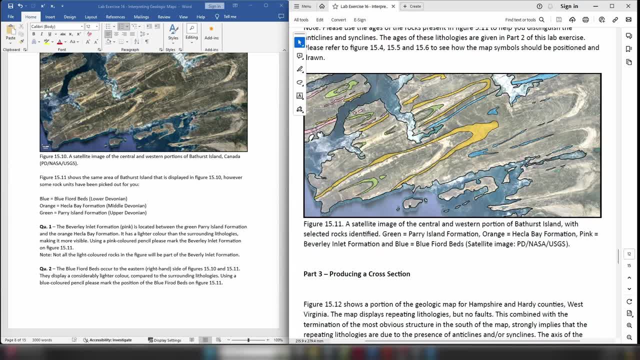 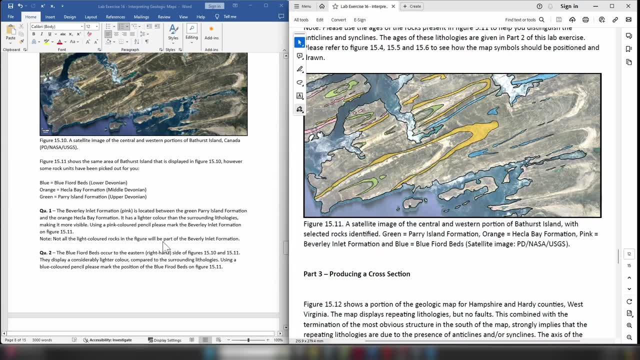 the youngest. This is going to be important for when you try and work out whether these features are anticlines or synclines. Now for question one. I've also picked out an additional formation. So this is the Parry Island formation and this is upper Devonian. So the blue rocks, the rocks I've 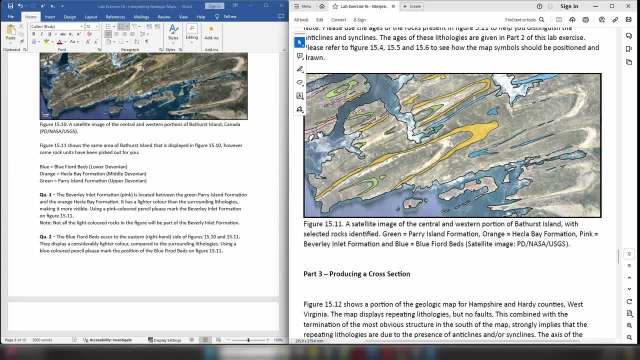 picked out in blue is the Beverly Inlet formation, and this has been picked out in pink and you can see it here up here here. So there's a few locations where I've already picked it out for you Now. the Beverly Inlet formation is located between the green Parry Island formation and the 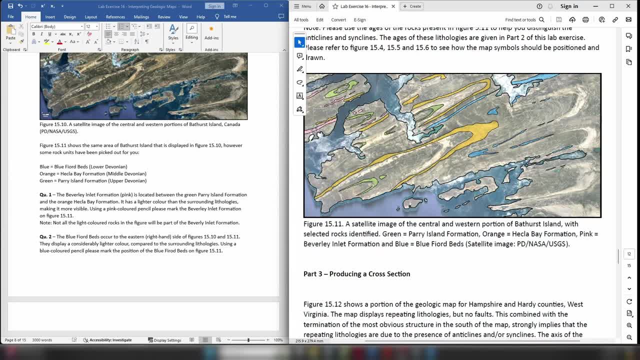 orange Hekla Bay formation. So this green layer here is the Parry Island formation, and the orange layer here is the Hekla Bay formation. So this green layer here is the Parry Island formation, and so the Beverly formation will be located between these two layers of rock. And I also point: 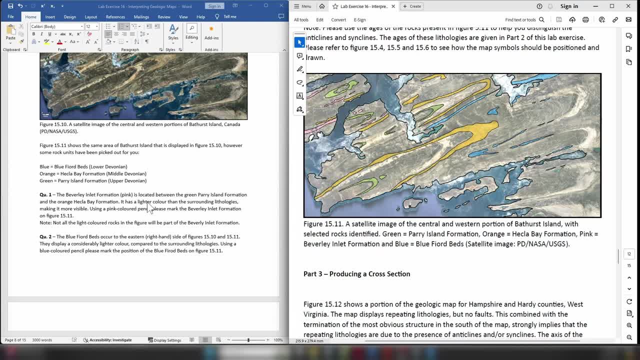 out that it has a lighter colour than the surrounding lithologies, So this pink layer of rock is probably going to be visible in our satellite image. So, when we are looking at our satellite image, here's the Hekla Bay formation. Here is the Parry Island formation. 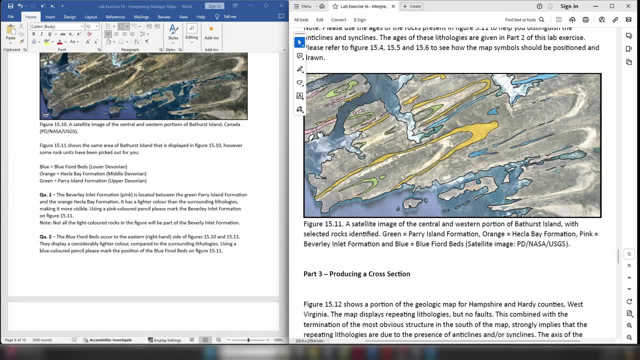 So we know that the Beverly Inlet formation is going to be somewhere in this area, here between these two layers, and we know it has a very light colour And so when you look at this satellite image for this feature in particular, you can probably pick out that layer of rock quite easily. 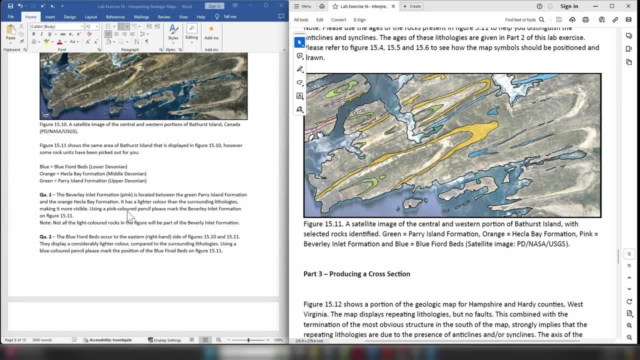 So, once you've picked it out, you are going to colour it in using a pink coloured pencil. Now remember, we are looking at an area that has been deformed and it's produced anticlines and synclines. This means that we are going to see: 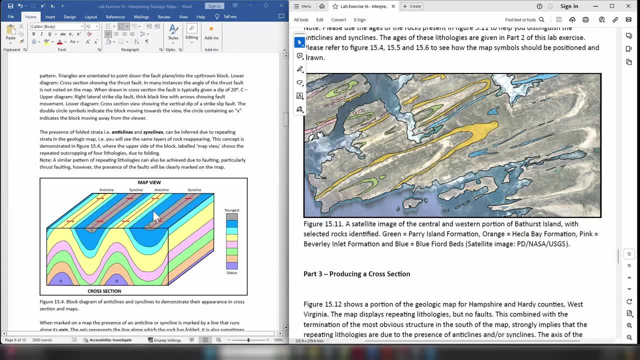 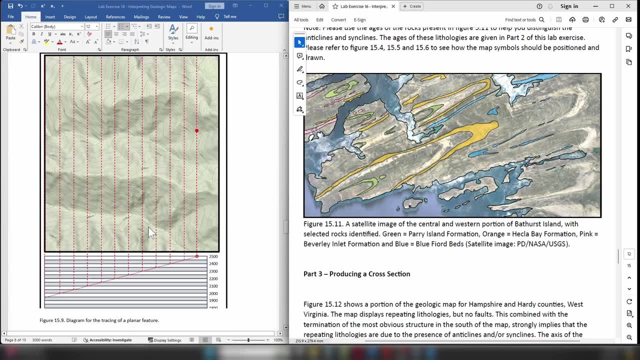 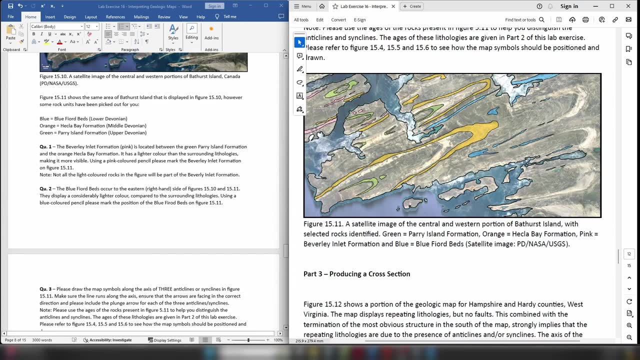 the same layers of rock repeating at the surface. So the Beverly Inlet formation isn't just going to appear in one of these anticlines and synclines. There is a very good chance that it's going to appear in more than one. So we have one anticline or syncline here and then we're going to move on. 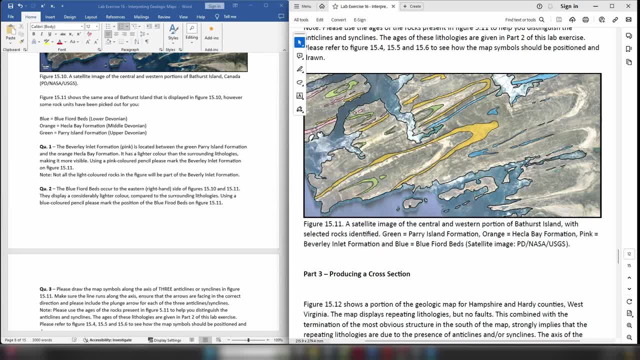 to the next one. So once again, we're going to pick out the Hekla Bay formation and we're going to pick out the Hekla Bay formation picked out in orange. Here is the Parry Island formation picked out in green, And then we know that between those two formations is going to be the Beverly Inlet. 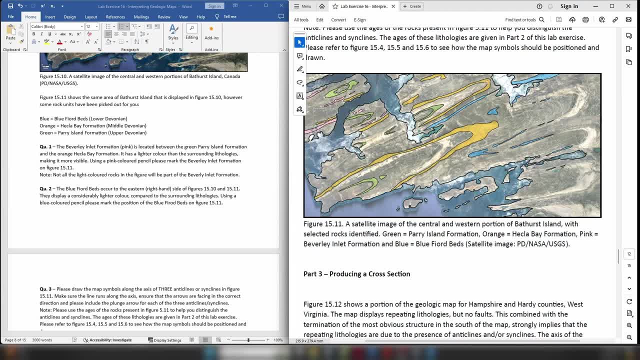 formation. And so, once again, look for that light coloured layer of rock between these two formations. And, you know, you may even be able to pick out other locations where you see the same thing. So, for instance, you could say that maybe this sweep of lighter coloured rock here, 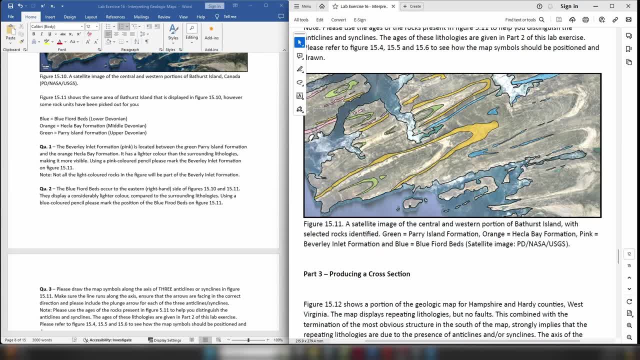 is also the Beverly Inlet formation because it would be located between the Hekla Bay formation right here and the Parry Island formation located right here. Now to be clear, though, not every light coloured rock is going to be the Beverly Inlet formation, So over here you can pick out. 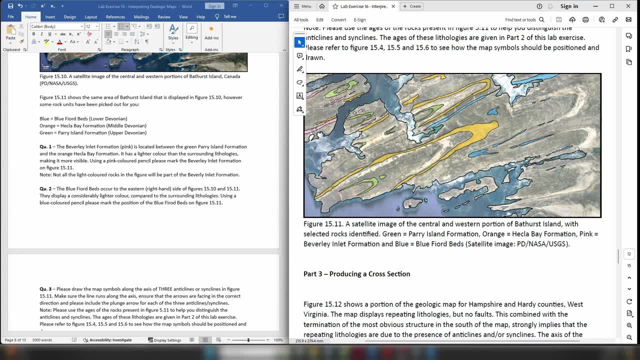 light coloured rocks as well. However, they are not the Beverly Inlet formation because we know they are not the Beverly Inlet formation. So we know that they are not the Beverly Inlet formation because they are not located between the Hekla Bay formation and the Parry Island formation. 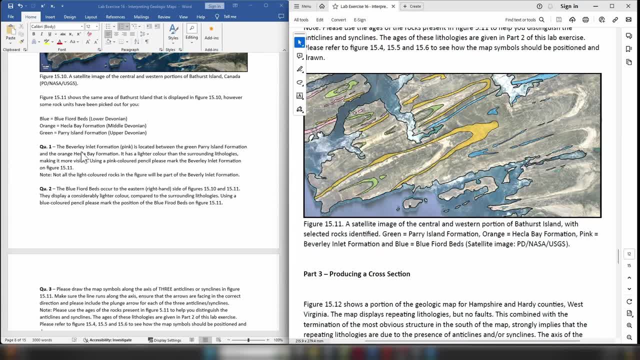 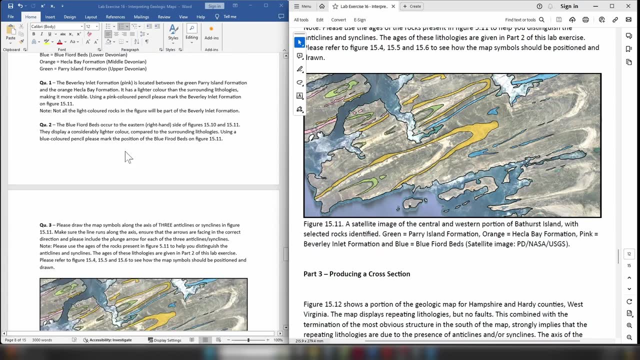 Okay, so for question one, you are going to be picking out the areas where the Beverly Inlet formation is exposed And you're going to be marking those with a pink coloured pencil or pink highlighter. So on to question two. So for question two, we are going to be looking at the 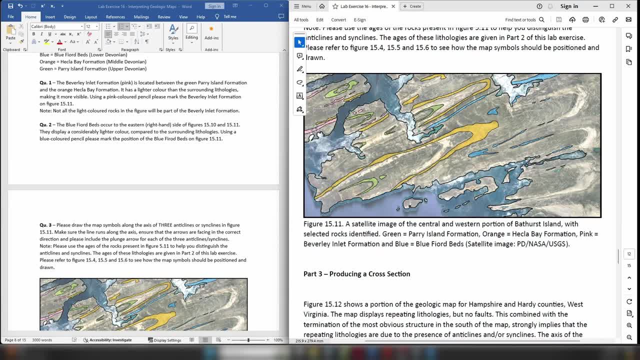 blue fjord beds And these are picked out here in this light coloured rock. So for question two, you are going to be looking at the blue fjord beds And these are picked out here in this light blue colour, So you can see some here. There's some outcrops here, a couple there, And you can 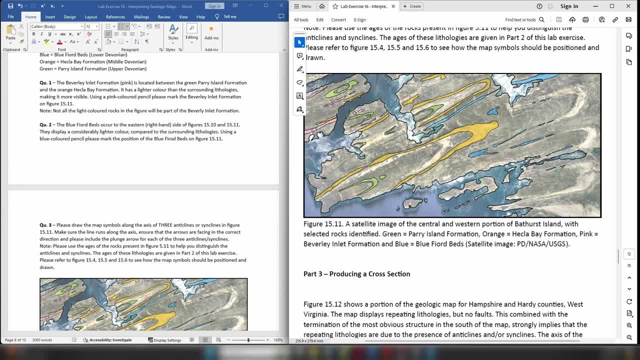 see the sweep of an anticline or a syncline here. You can see it comes around. We have them here. We can see we have another feature here as well. We can see one side of it there, one side of it here. So the blue fjord beds are occurring on the right hand. so eastern side of our satellite image. 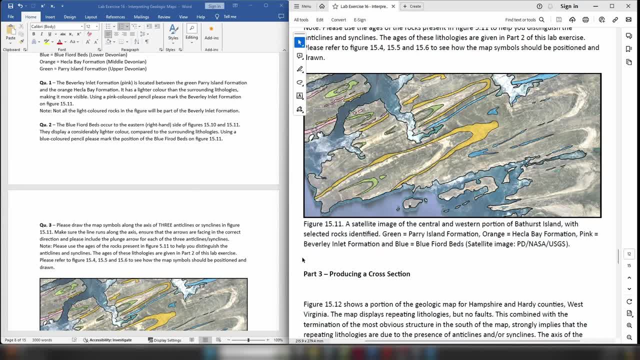 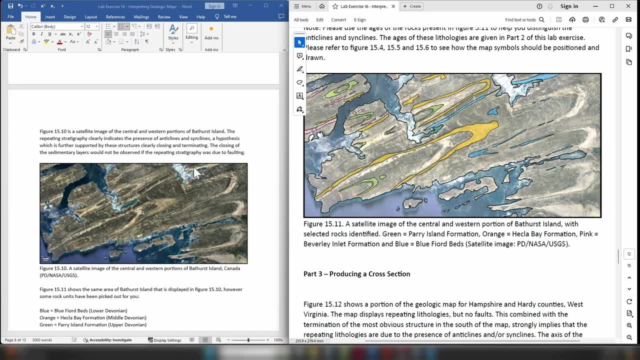 And we can spot them quite easily because, as you can see, if we look at the original satellite image, this is the blue fjord beds right here. They once again have a much lighter colour than the surrounding area And they are clearly more resistant to erosion. 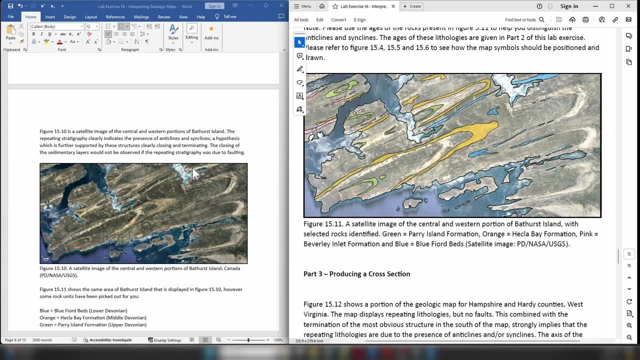 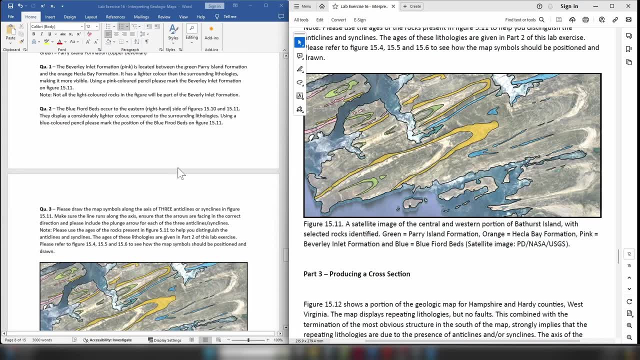 because they're forming topographic highs, So you can see them relatively easily in the satellite image. So for question two, you are going to be doing exactly what you did in question one, but you're going to be doing it for the blue fjord formation. 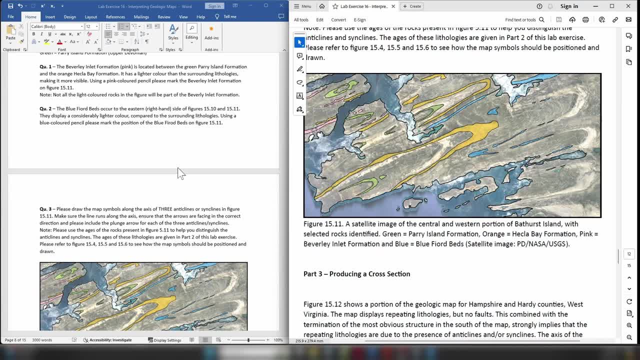 And so you are going to be picking out the blue fjord beds with a blue coloured pencil or a blue highlighter, And so you know, the area of interest is over here on the eastern side of our diagram. Okay, so any of these lighter beds over here on in the central and western portion. 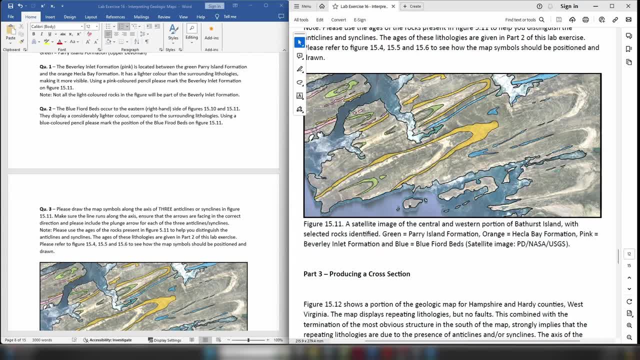 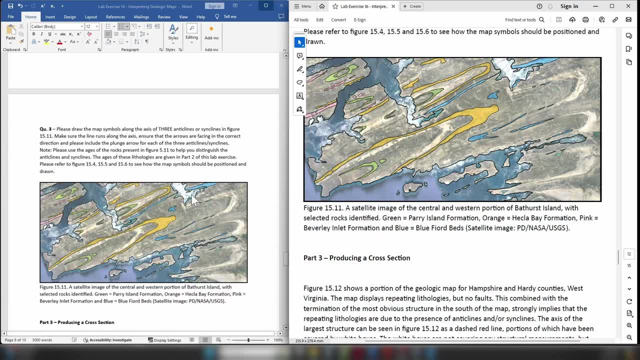 those are not part of the blue fjord beds, So ignore those. Okay, so for question two, you're going to pick out where the blue fjord beds are going And then, in question three, you are going to pick out where the blue fjord beds are going, And then in question three: 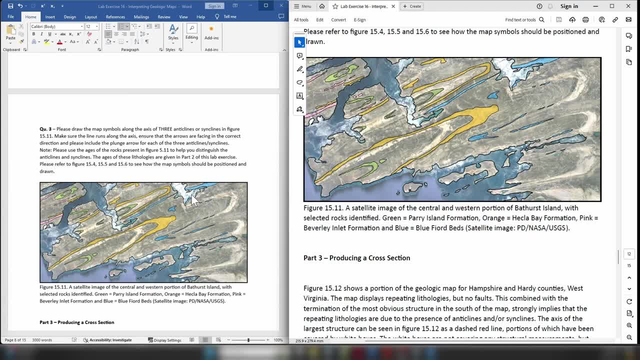 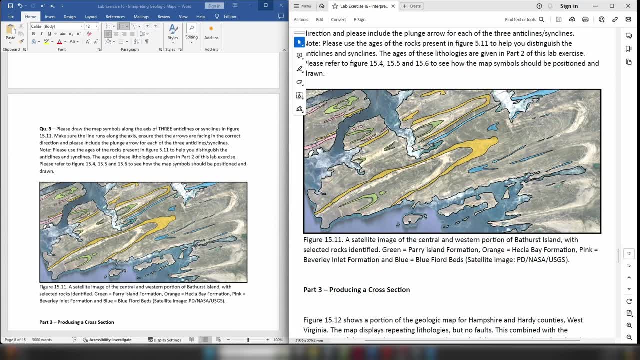 you are going to draw the map symbols along the axis of three anticlines or synclines. All right, so you're going to look at this map and you're going to say, right, well, I clearly have one feature here, because I can see it closing up and coming back round. So 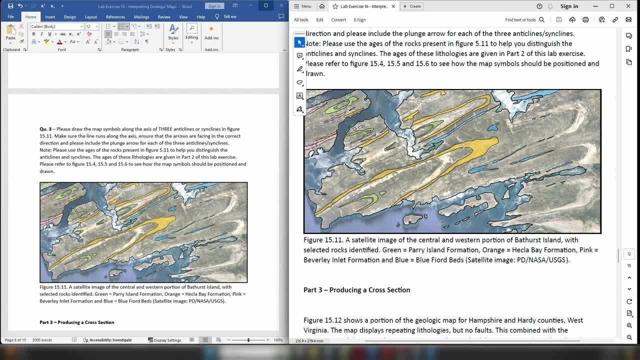 I've got one axis here, I've got another feature right here, So I've got another axis coming through here, like that, And then maybe you've got this feature here which is sweeping round. So you know, you have another axis coming through. 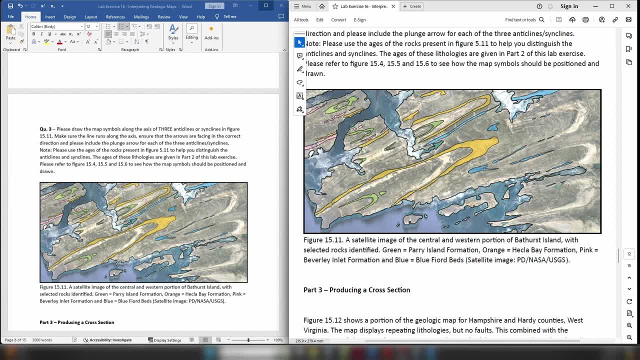 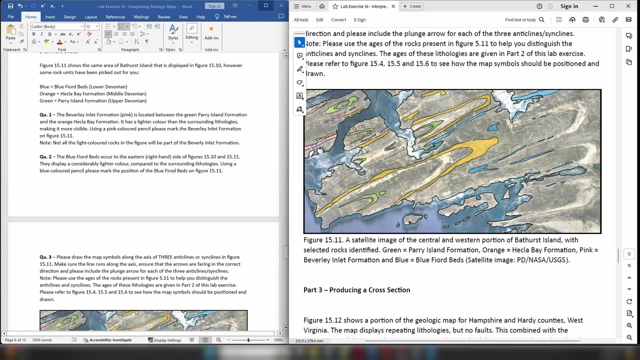 Here. So the question is going to be: what are they? Are they anticlines or are they synclines? And, as we've already touched on, the way to do this is to look at the ages of the rocks. So when we look at our map here, we know that the blue fjord beds which are picked out in blue 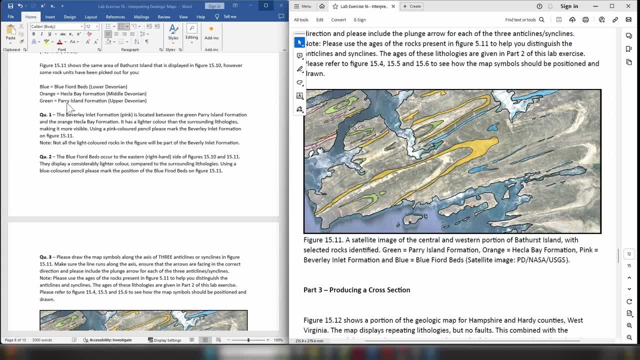 are the oldest And the Parry Island formation picked out in green are going to be the youngest of the Devonian. So we know that this is going to be the youngest and these are going to be the oldest. So that should allow you to work out whether you're looking at an anticline or a syncline. 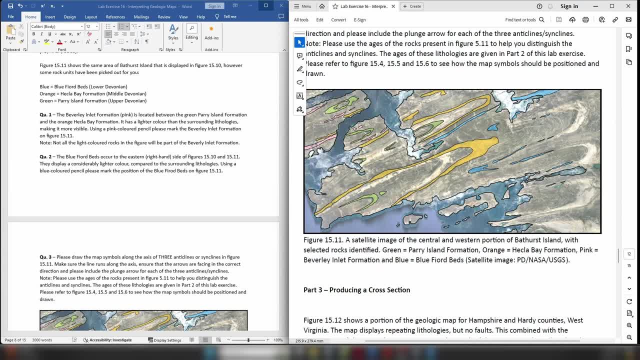 And so you're going to mark out the axis for three of these features. So if we take this larger feature right here, we know that the axis itself is clearly coming through here, through the point of this folded green layer here. So we're going to come up. 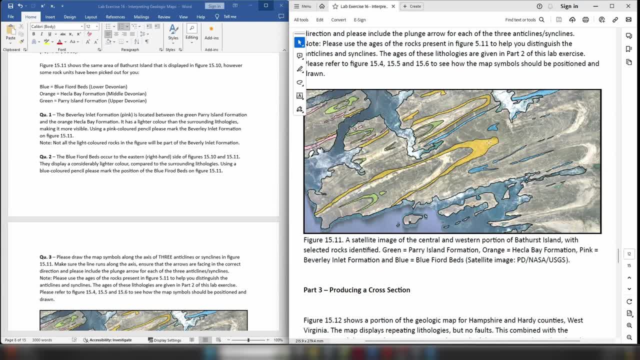 The axis is then obviously coming through this region here because we can see the hinge right there, And then it's going to continue up here through this feature because once again we can see another hinge region right here. So our axis is going to come all the way up through here, like so. 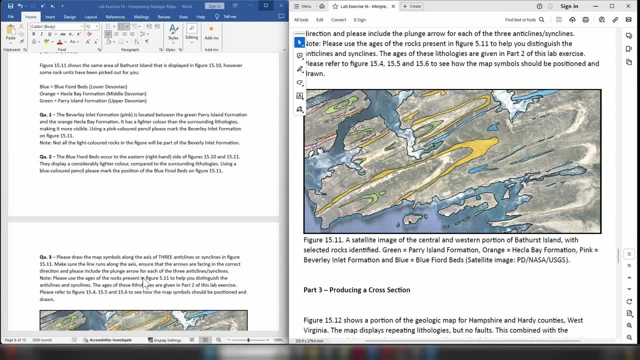 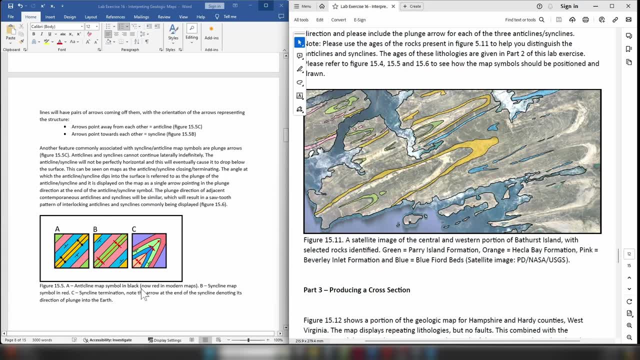 And the final thing you're going to have to do, though, is you're going to have to use the correct map symbol to denote whether it is an anticline or a syncline, So that's going to require you to to return to these diagrams right here, and obviously we have the map symbol for an anticline. 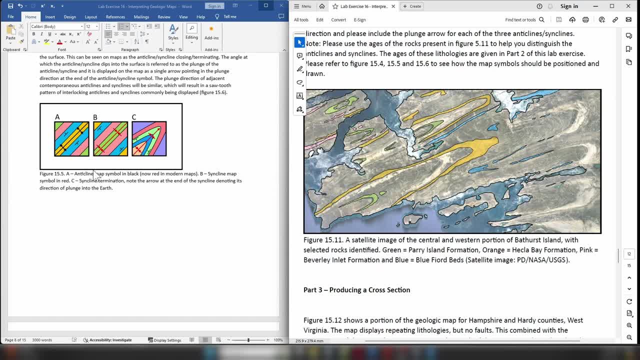 and the map symbol for a syncline, and so you're going to use the correct map symbol to say: right, this feature is an anticline or syncline, and once you've drawn the axial trace showing where the anticline or syncline is going, you're then going to add the arrows coming off that line or going. 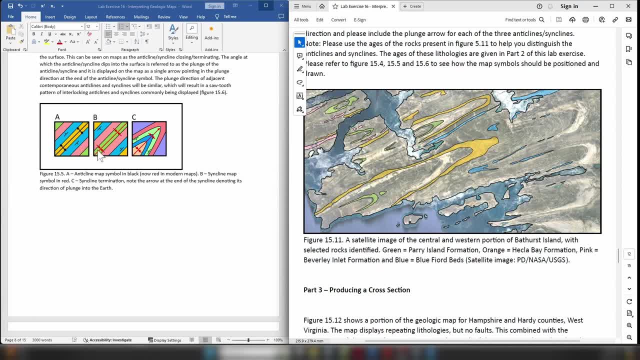 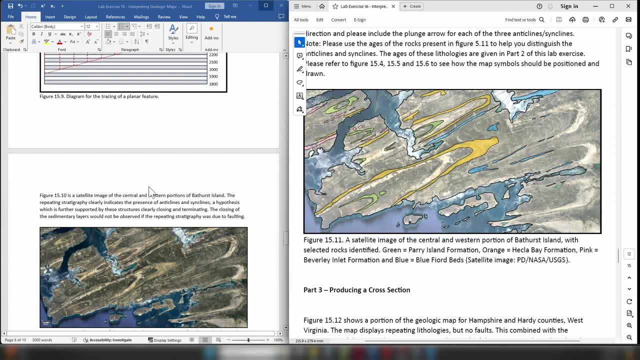 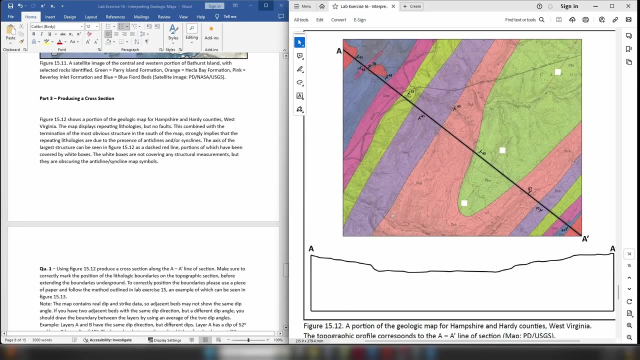 towards that line to tell me whether it's an anticline or a syncline. okay, so now we are going to be moving on to part three. so part three is going to be dealing with this map right here. so you can see we have a geologic map. you can see it's been overlaid on a topographic map. you can. 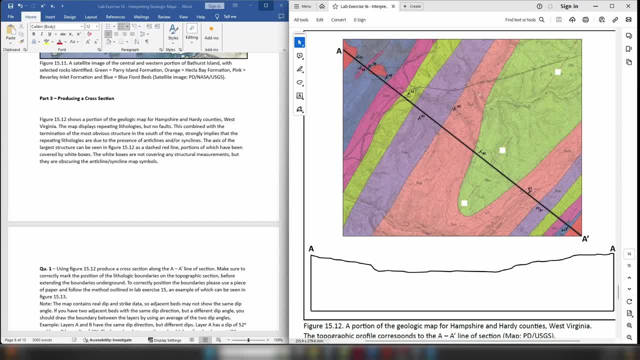 see the contour lines quite clearly and you can see that we have a situation where we have repeating stratigraphy. so, for instance, we can see we have red where this red colored rock, here, there and there and here we have this dark blue, there and there we have this kind of hot pink. 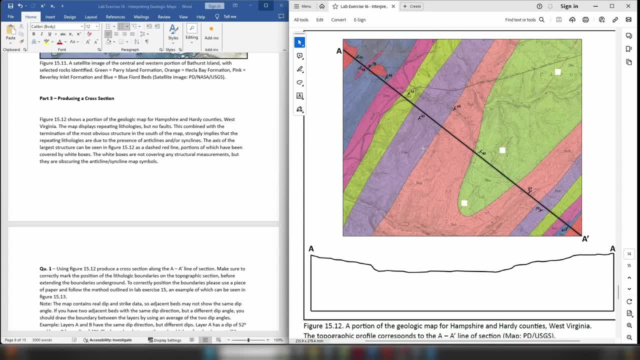 there and there. we have this slightly neon green there and there, we have this purple there and there, and we have this peach colored rock here and here. so we have repeating stratigraphy straight away. we're going to be thinking: right, this is either due to a fault or a fold. what could it be? 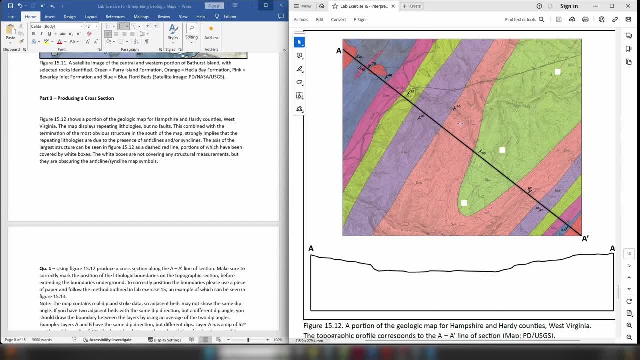 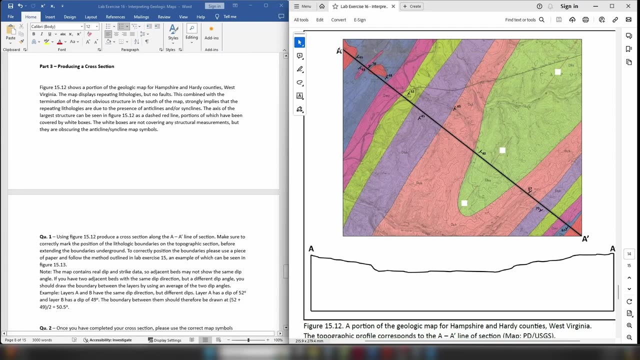 well, straight away, there's no indication of any faults on the map. so this instantly begins to suggest that what we're looking at is either going to be an anticline or a syncline. so okay, so for part three we are going to be drawing a cross section. it's going from a to a prime and 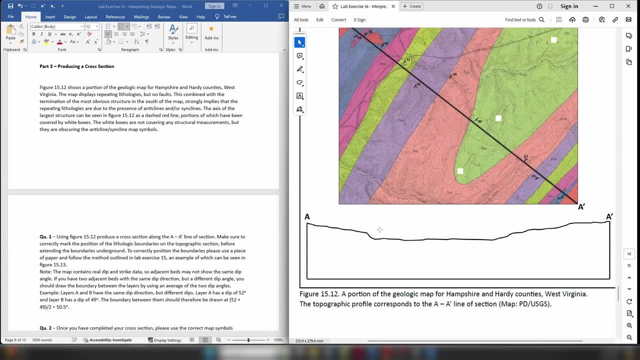 you will see, the topographic profile is given directly below the geologic map. now, in this instance, you will notice that the topographic profile is not orientated parallel to the line of section on the map. this means that you cannot just say, right, that's where the boundary crosses. 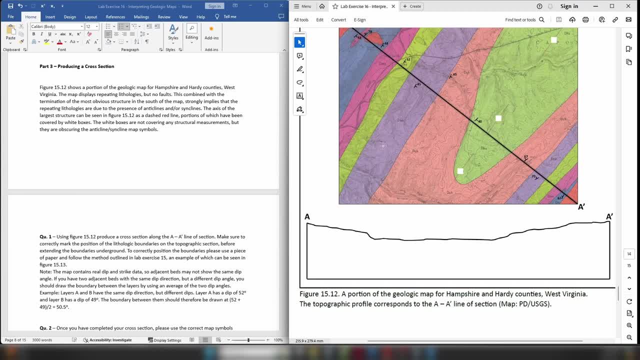 the line of section right here, i'm going to draw a vertical line straight down and i'm going to mark the boundary position right here on the topographic profile. no, you cannot do that. remember, you can only do that if you have a topographic profile and you have a topographic profile. 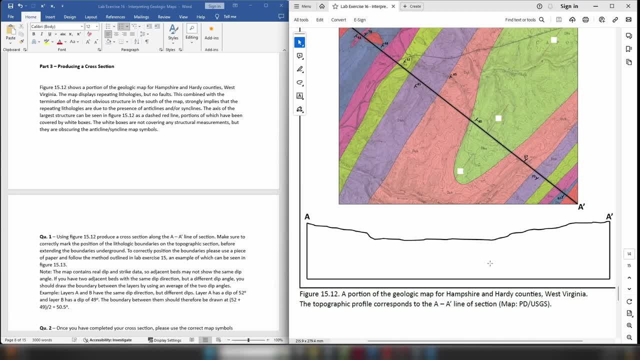 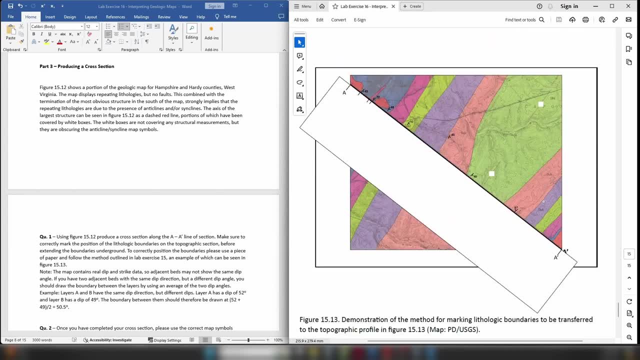 so you can only do that when the line of section and the topographic profile are running parallel to each other. in this instance they are not. so in this case you are going to have to use the paper method. so you're going to take a piece of paper and on that piece of paper you're going to line. 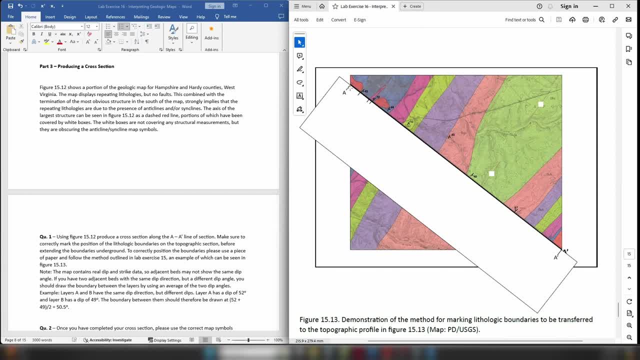 the straight edge along the line of section and you're going to mark the start point as A and the end point as A-prime, and then along this straight edge, you are going to mark off every point, so any locations where a contact hits the line of section. so you're going to put a mark here, here. 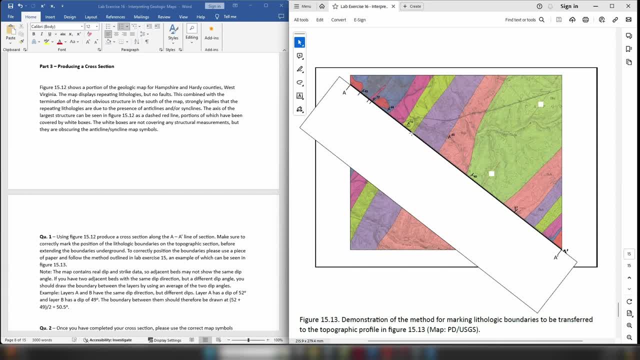 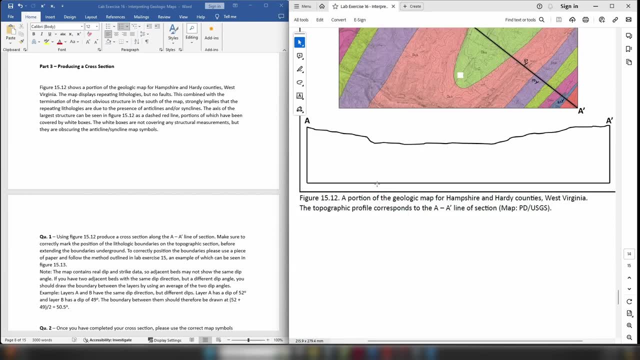 here, there, there, there, there, there, etc. all the way along the line of section, and you can then take this piece of paper and you can then put those points onto the topographic profile so you have the locations for each of the boundaries on the surface correctly marked on your topographic. 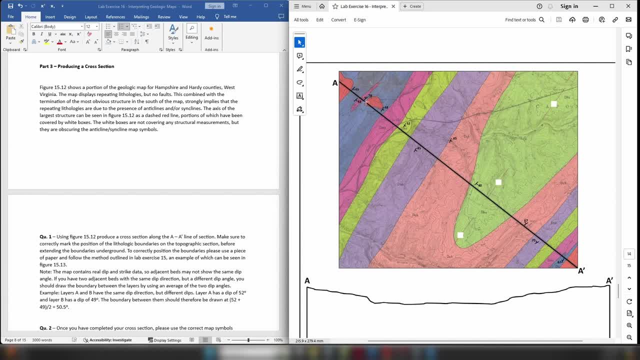 profile. you will then also see that you have several dip and strike symbols. you will notice that, because this is real data, the dip angles are not consistent. so for instance you can see: here we have a dip of 48, dip of 52, 45, 45, 40, so you can see the dip angle is changing between these. 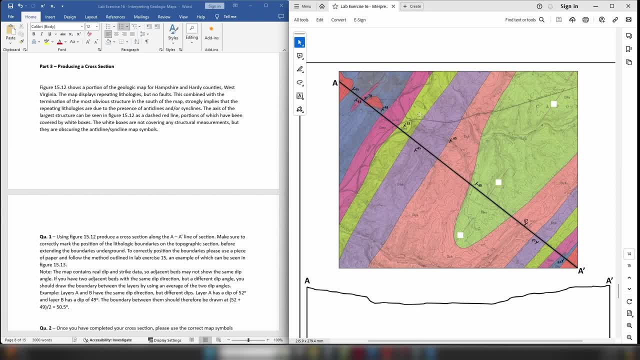 locations once again, as you did in previous labs. so, for instance, you can see: here we have have a dip of 52, here we have a dip of 45. when you are drawing this boundary between them, you are going to take the average between those two dip values to draw this boundary. here, in the case, 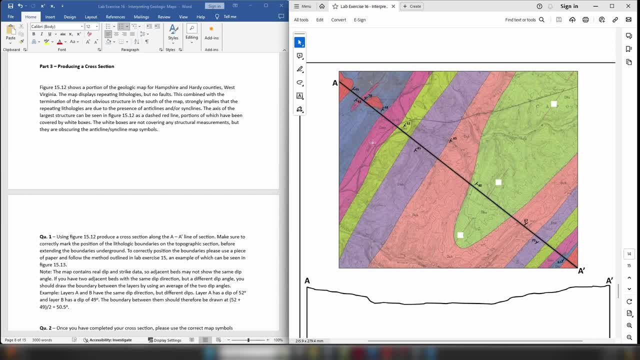 of this pink layer, you will see that there is no dip or strike symbol associated with it. but we can infer the dip and dip direction for this layer rock by looking at the layers above and below it, so you can see. to the west of it we have this blue layer and this has a dip of 48 degrees. 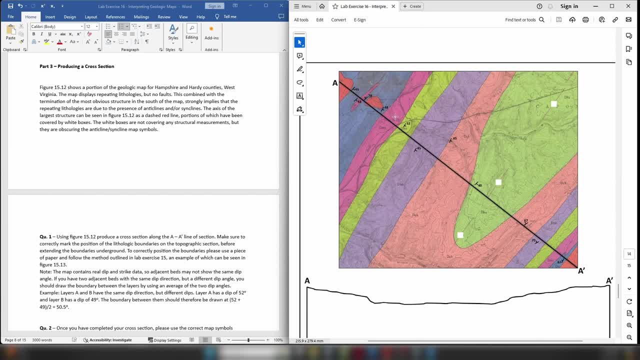 towards the southeast. in the case of this layer, this kind of neon green layer- here you can see, you have a dip of 52 degrees, once again towards the southeast. so when you draw this pink layer, this lower boundary, you are going to be drawing at 48 degrees and this upper boundary is going to 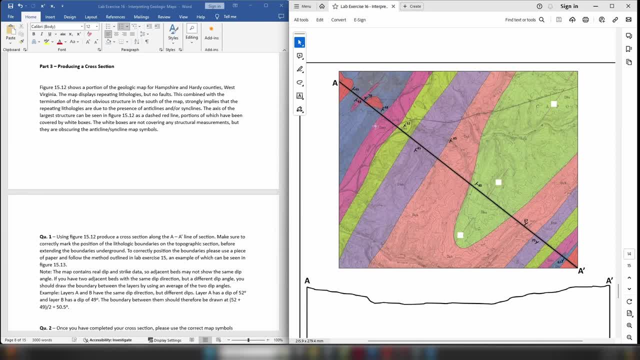 be drawn at 52 degrees. all right, no averaging. in this case, you're going to say: right, the lower boundary is going to be angled at the same angle as this outcrop here, and the upper boundary is going to be following this layer of rock right here, and so you are going to be drawing your cross section. 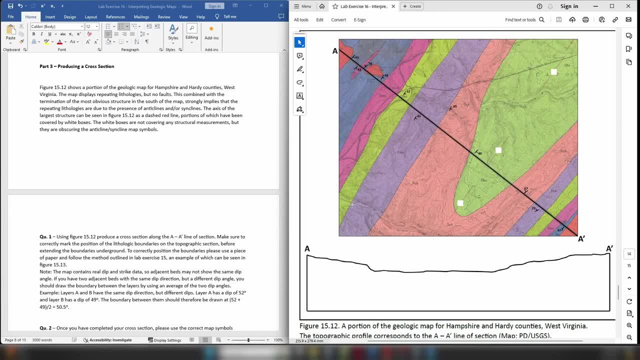 and, as previously touched on, this is probably an anticline or a syncline, and as soon as you draw your cross section, hopefully it should become pretty clear that you have a dip of 52 degrees towards the left of it. so we have a dip of 22 degrees across square cinema. this is obviously 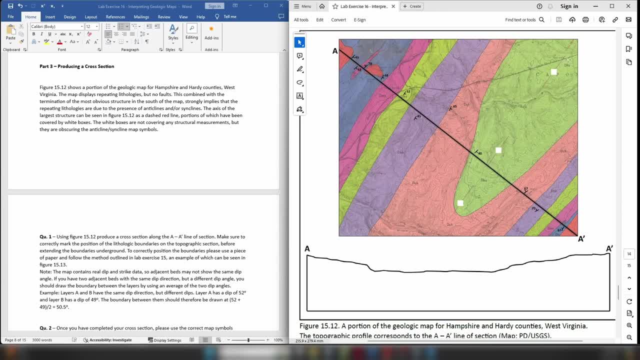 an anticline, but you need to note also that this is just the bottom part of the neither we talked about earlier. we talk about things of what we want to describe, and we can say plus two, and so these are kind of the points that should be referred to as the interlock points. 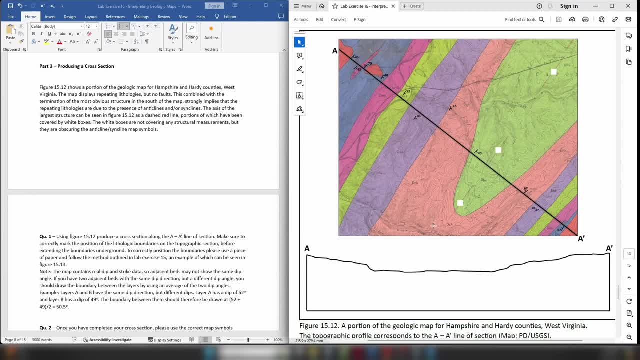 and so, without further ado, I just want to ask you to take the stage to which I've went into a zero balance into what I mentioned, that is, we're then going to go into adding strong. all right, let's introduce one more be. finally, I've shown you the center io. 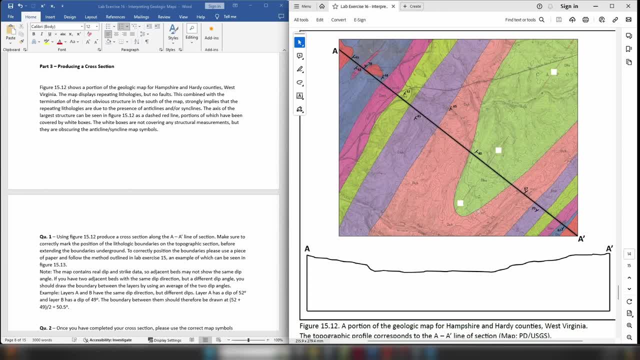 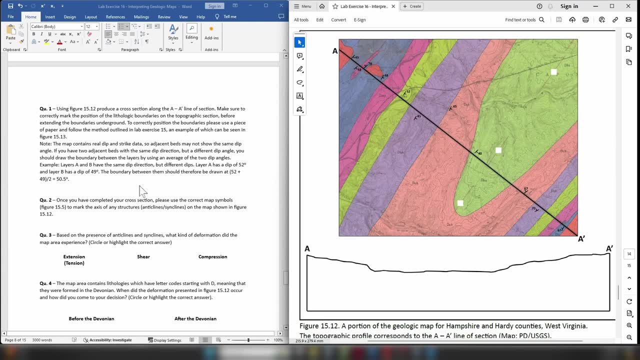 here we've actually done the dimension method, which is that of giving an inner ongoing of structure. it is so, for figure for question one, you are going to be producing your cross section, and then for question two, once you've completed your cross section, please use the correct map. 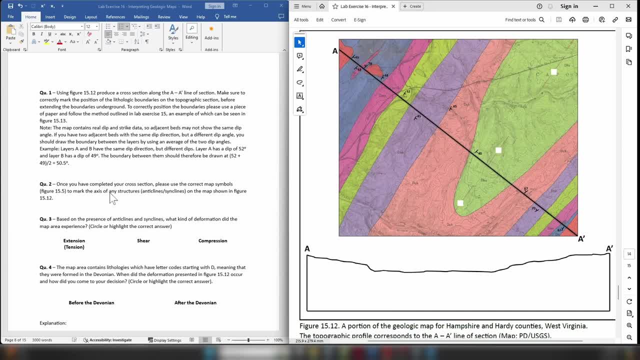 symbols on this figure to mark the axis of any structures: anti-clines and sync lines. so this is the point. so for question two, this is when you're going to draw the arrows on the map telling me whether it is an anticline or a syncline, and of course that is going to be based. 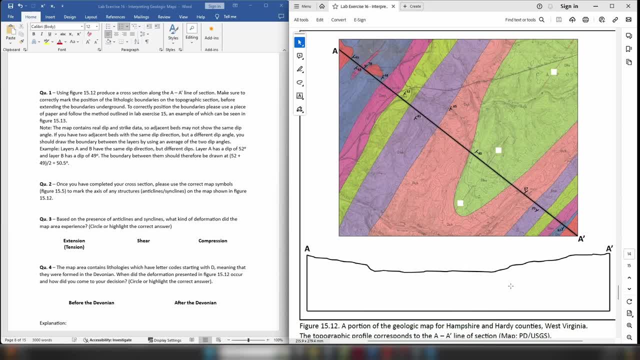 on your cross section. i would also point out one thing you are. you can quite clearly see one very large anticline and syncline right here. however, that is not the only one on the map. if you look up towards the northwestern corner, you will actually see there is another feature, so you will be. 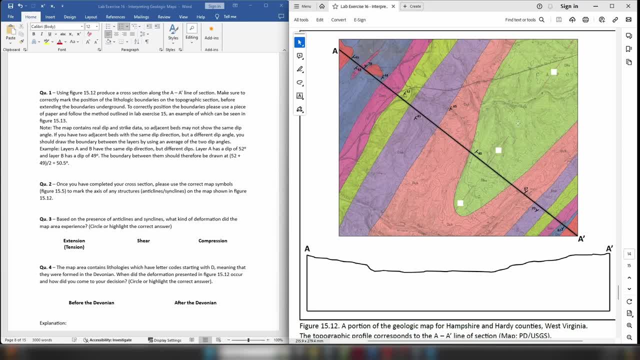 drawing the axial trace for this anticline and syncline. but there is also another, smaller anticline and syncline towards the northwest, for which you will also be marking the axial trace of it and providing the arrows telling me whether it is an anticline or a syncline. so then, for question three we are. 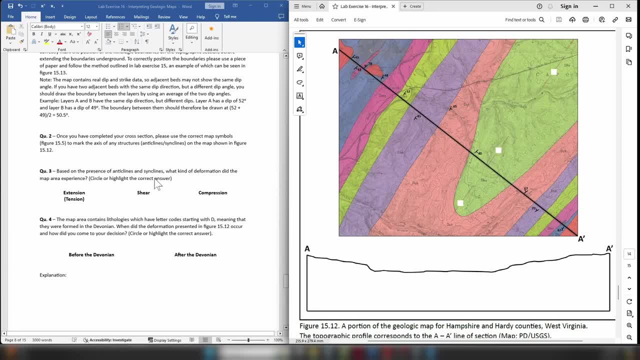 going to start thinking about possible causes for this deformation, and we're going to do this because this is going to be the kind of thing we're going to be looking at in the next video. Thanks, and have a great day. lab exercise. So for question three, it asks you, based on the presence of the anticlines and 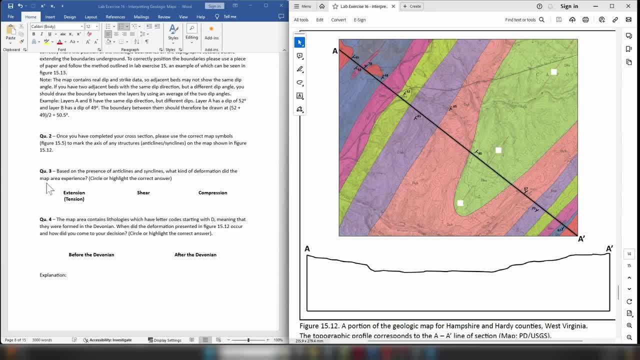 what anticline and or syncline? what kind of deformation did the area experience? So was it extended? so was it stretched? Was the area sheared or was the area deformed due to compression? So what kind of compression caused the formation of these anticlines and synclines? Extension, so the